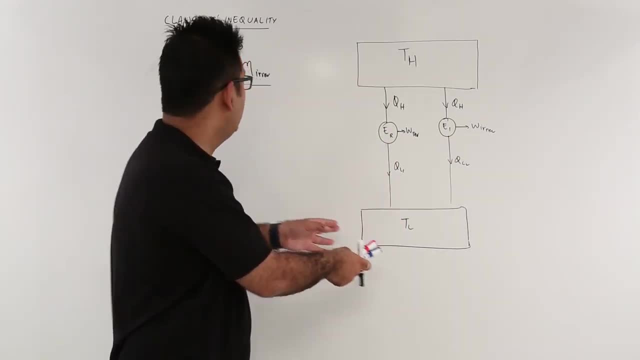 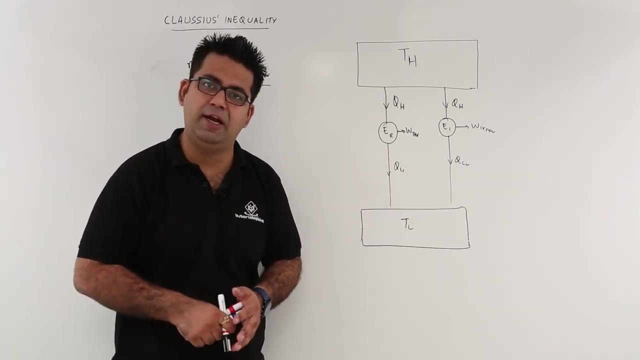 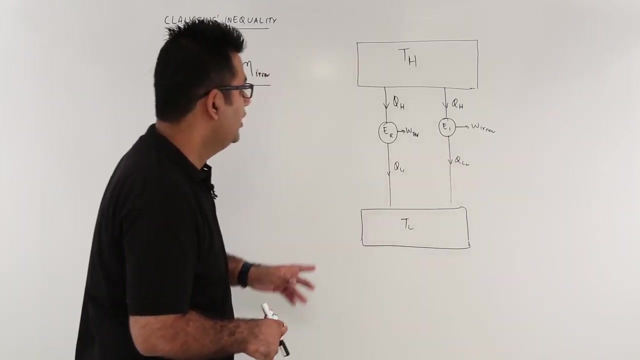 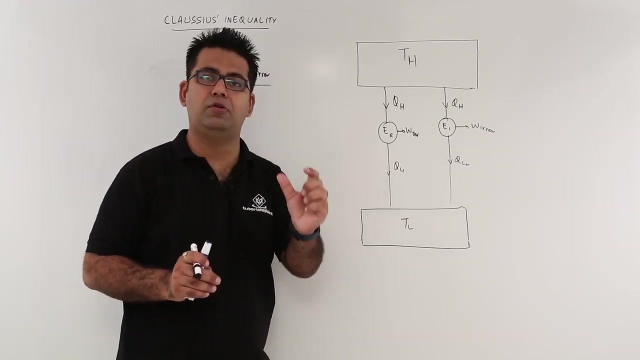 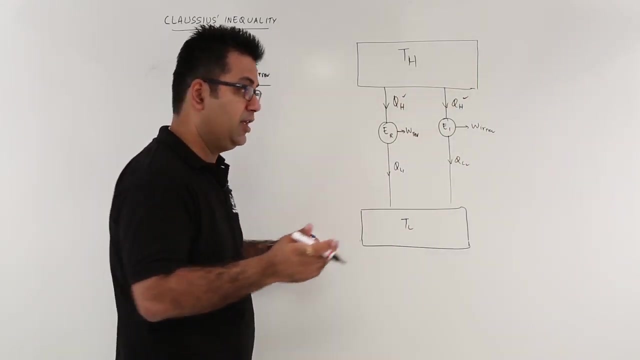 And the same is true for a heat pump. So for a reverse Carnot heat pump, you would have the maximum possible COP against all irreversible heat pumps. Okay, So you have this. You have this reversible heat engine and then you have an irreversible heat engine. Now they are working under the same temperature limits- TH, TL. Okay, We are giving them the same amount of heat supply, So this CO is the same. I will look over here, Okay, But obviously they are different engines. So this gives a reversible work output and this gives an irreversible work output. Okay, Now, due to this difference in the work output, we have to take a look at the example. 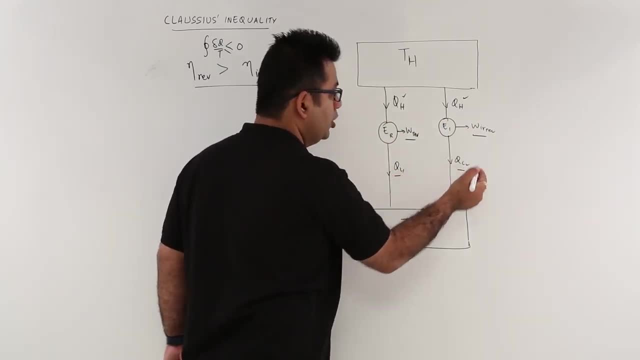 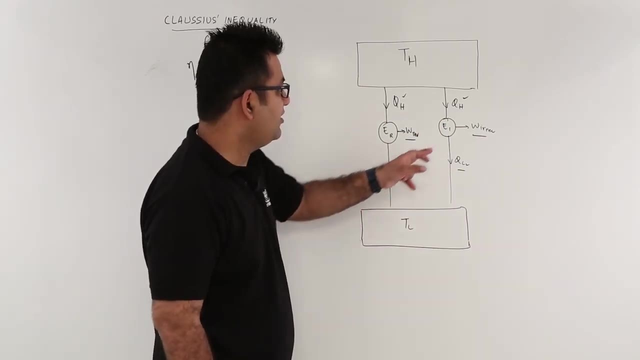 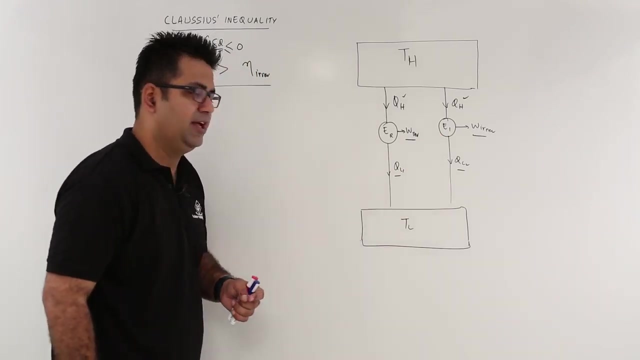 Okay, difference in the work output. you have different values of heat rejections. so the reversible engine is rejecting heat ql1 and the irreversible engine is rejecting heat ql2. okay, let's have a look at that for the- you can say- reversible engine. first of all, now the reversible engine. 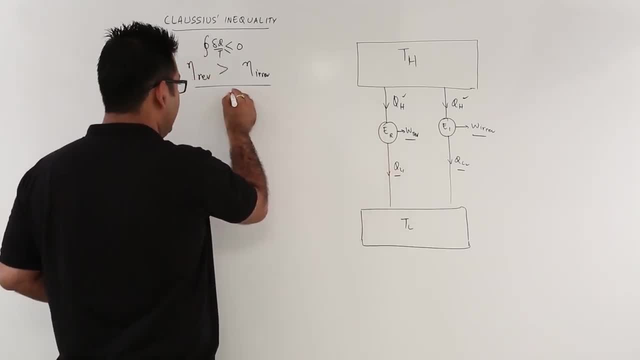 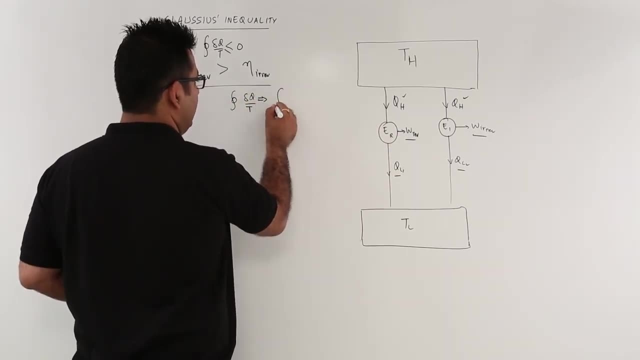 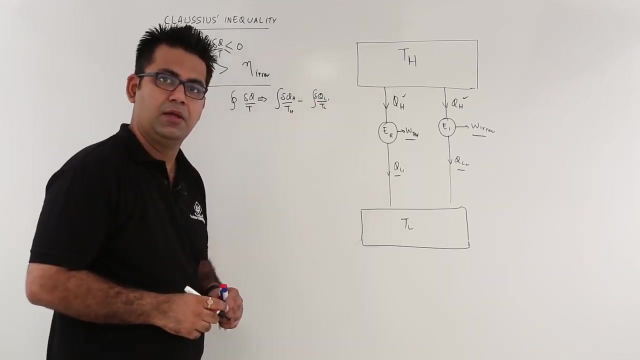 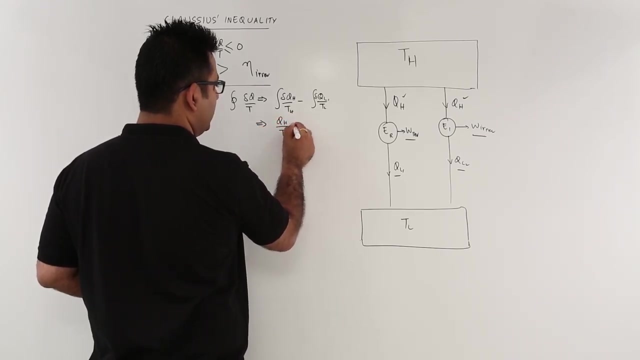 if i take the case, because it's a cyclic engine, if you take this part, okay, this is equal to integral delta qh upon th minus delta ql, this is l1 upon tl. okay, so this would become qh, TH upon TH minus QL1 upon TL. okay, so, because it's a reversible cycle, it's a reversible. 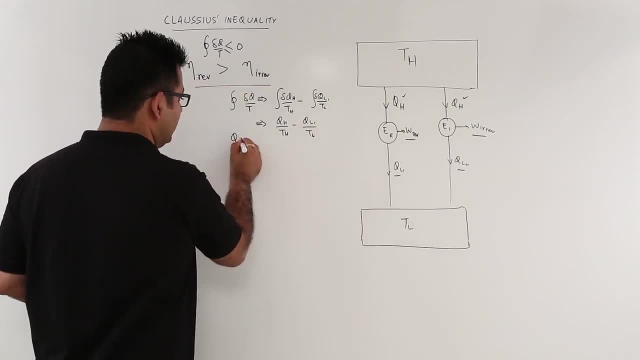 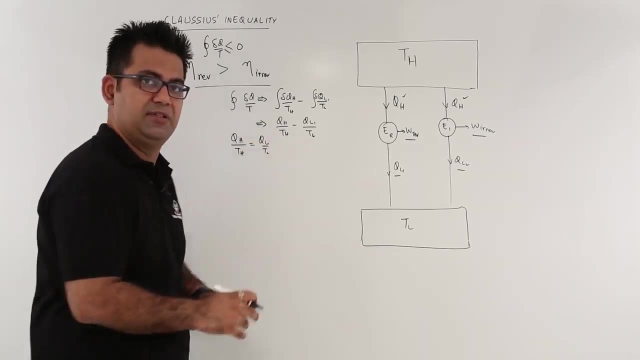 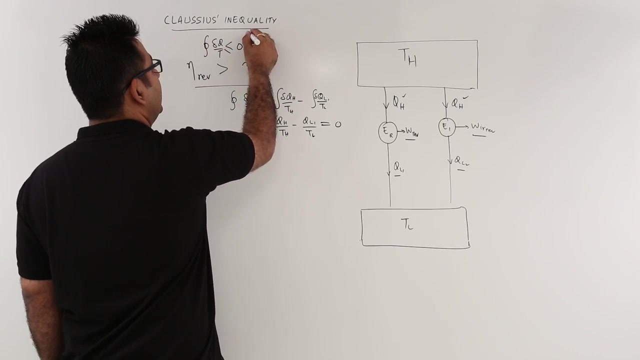 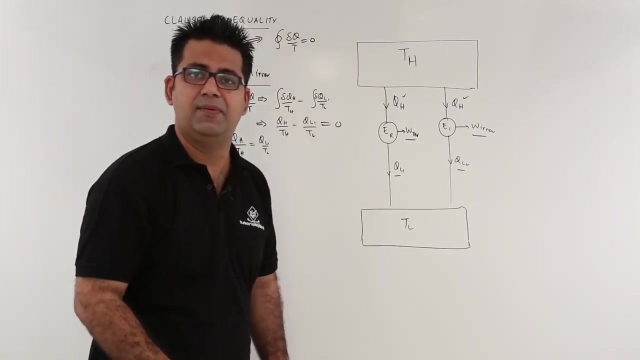 cycle. for a reversible cycle we always have this: QH upon TH is equal to QL1 upon TL. so this would be the case for a reversible cycle. so this would be equal to 0. okay, so from this, in equality, I can say that integral delta Q upon T is equal to 0 only for a reversible 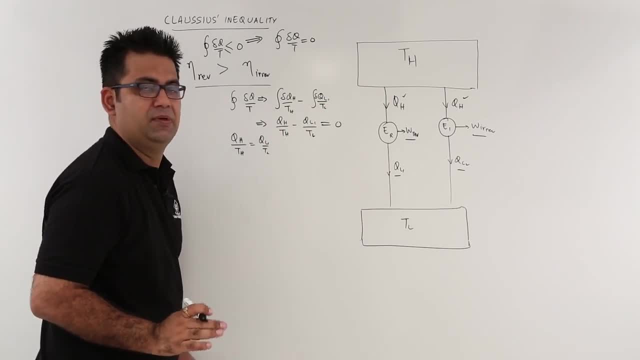 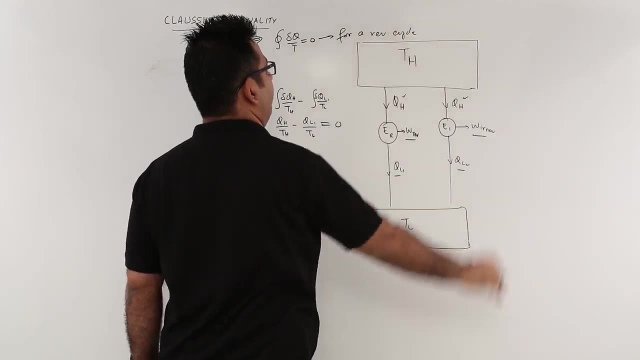 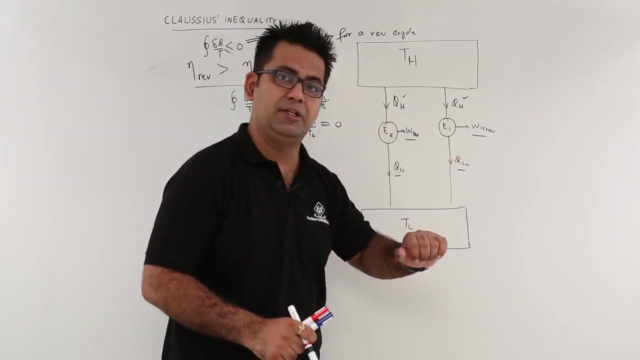 cycle. so this is proven for a reversible cycle. okay, so for a reversible cycle or reversible heat engine? okay, now let's come on to the second part, that is, the irreversible heat engine. okay, So if you look at this- because it is irreversible Inequality- I can say that integral delta Q upon T is equal to 0 for a reversible cycle. 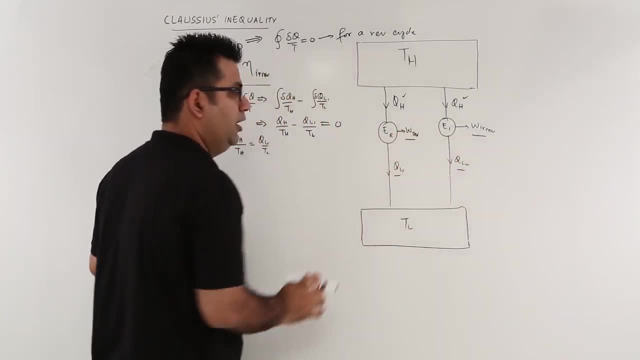 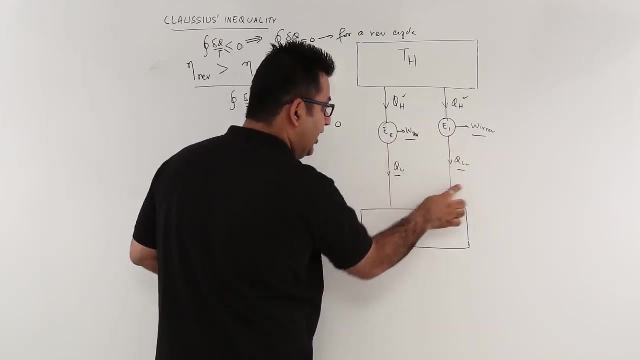 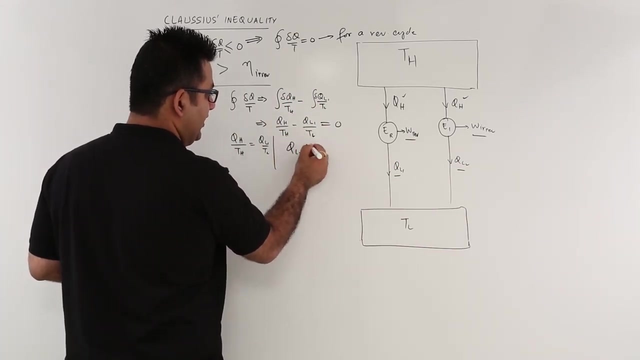 reversible, the work output would be less as compared to the reversible work output. so this means, because this is less as compared to this, the heat rejection would be more as compared to this. so we know that QL2 is greater than QL1 for obvious reasons. if I have to, 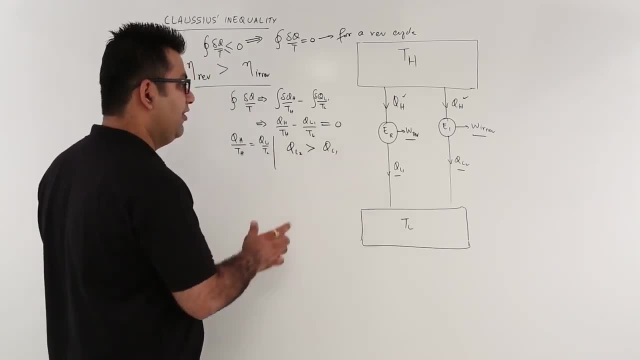 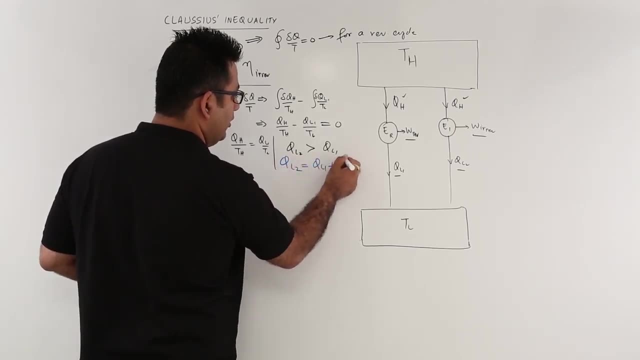 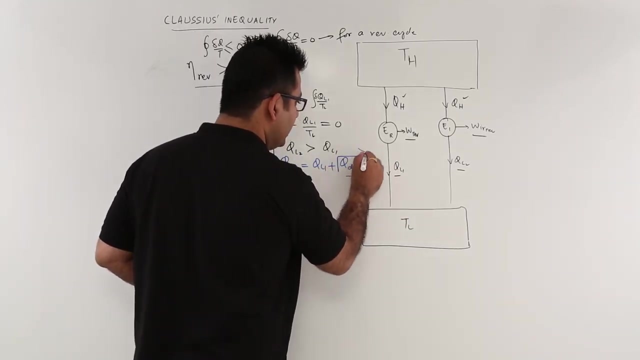 equate it, I will have to add something over here. that's the difference between the two heat rejections. so you would have: QL2 is equal to QL1 plus the difference in the heat rejections, and this particular value is always positive. this is never negative, okay, so let's apply. 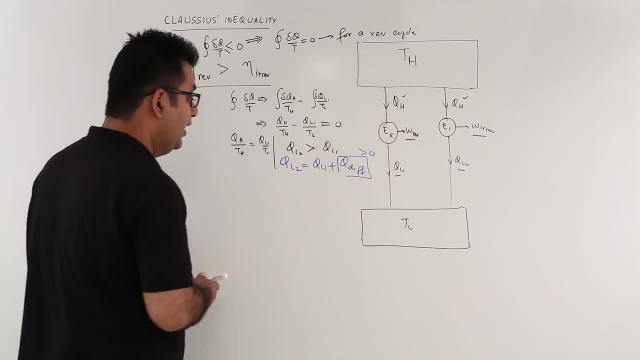 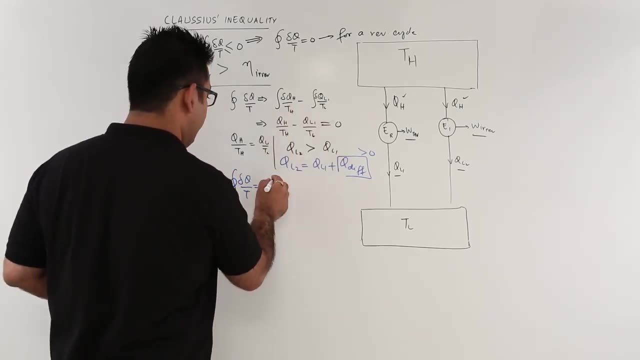 the same thing on to the reversible- you know irreversible- heat engine. so you will have integral delta Q upon T for irreversible. it would be integral delta Q upon T for irreversible, not the cyclic part, but only the integral, that is, delta QH upon TH minus delta QL2 upon. 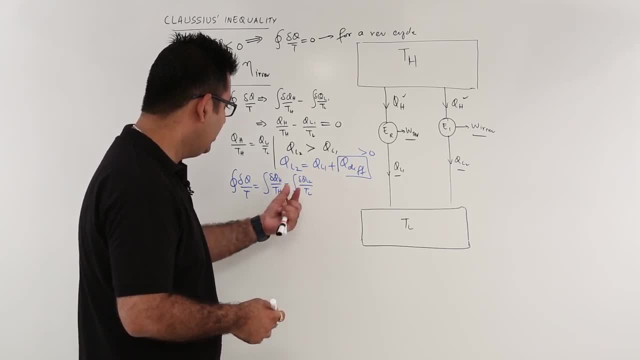 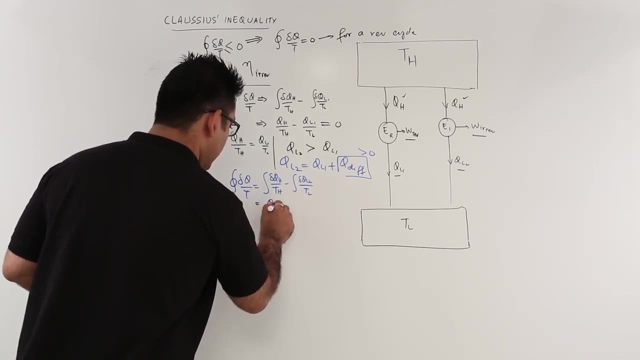 TL. now putting the values of, you know, QL2. we will put that after integration is done. so this gives rise to QH upon TH minus QL2 upon T2. if you put that in bracket you will get ql1 upon th, tl. this is tl, and then plus q difference upon tl. this is what you get. 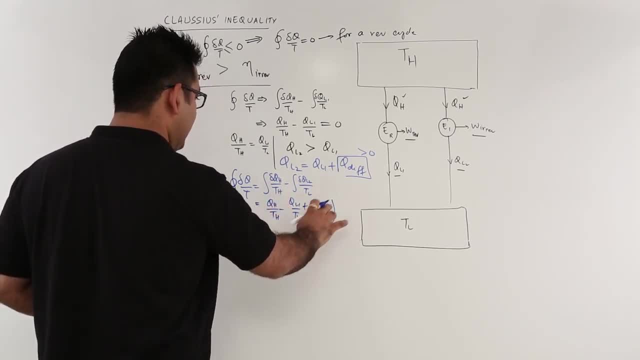 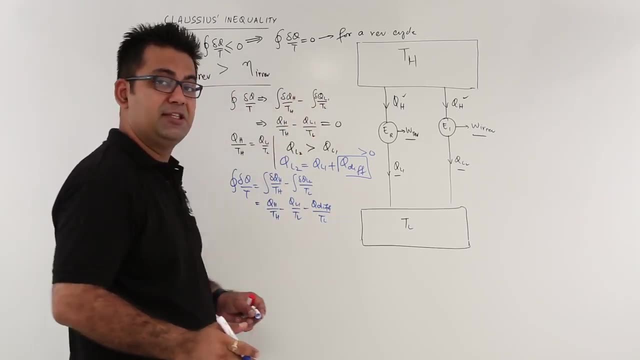 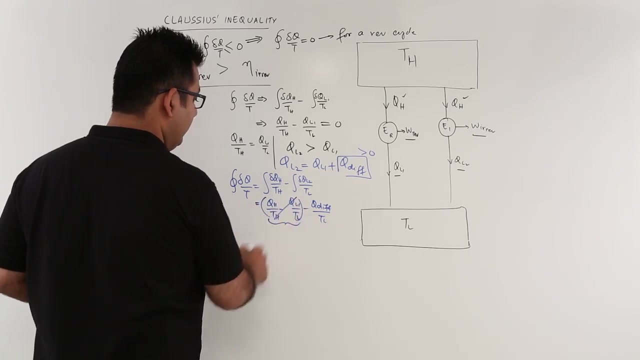 when you open the brackets. when you open the brackets, lets just get rid of these brackets. this would become a negative sign as well. now we know from our analysis of the reversible heat engine that this part is zero. ok, so this, these two things. it becomes zero because qh. 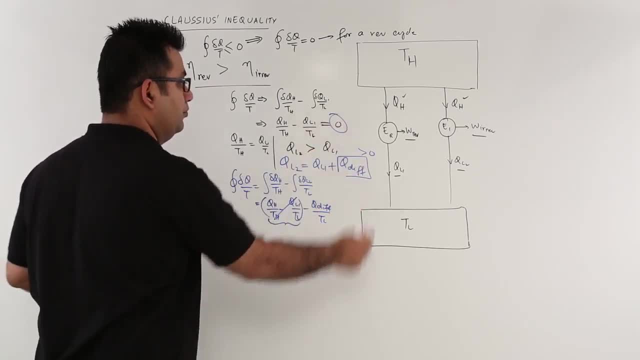 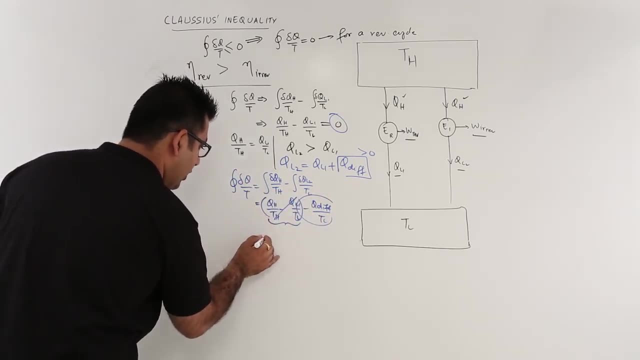 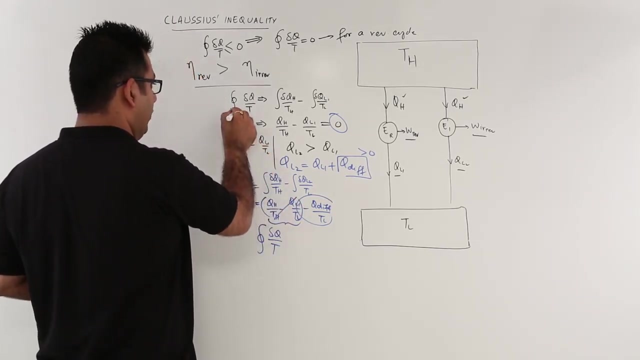 by th minus ql1 by tl is equal to zero. ok, so you are only left with this part. so you will get, let me write it down here, only so: delta q upon t. let me put something you know very important over here. so this is for reversible heat engine.